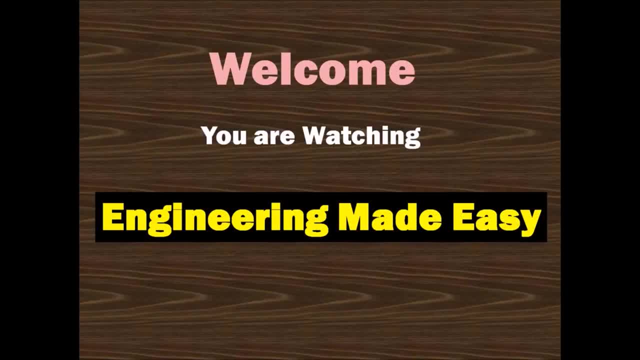 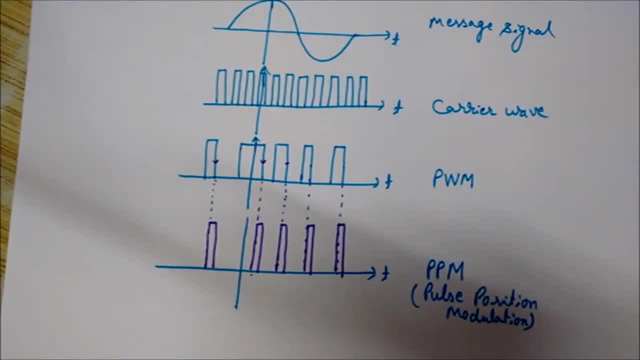 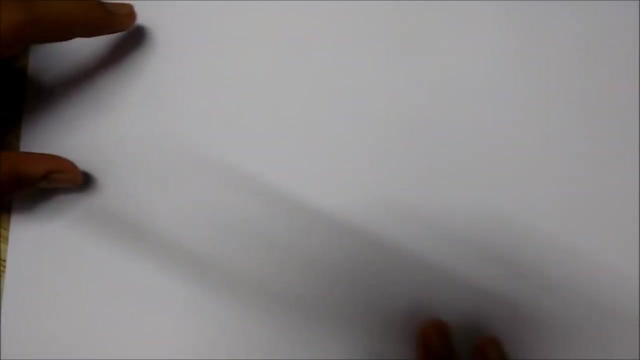 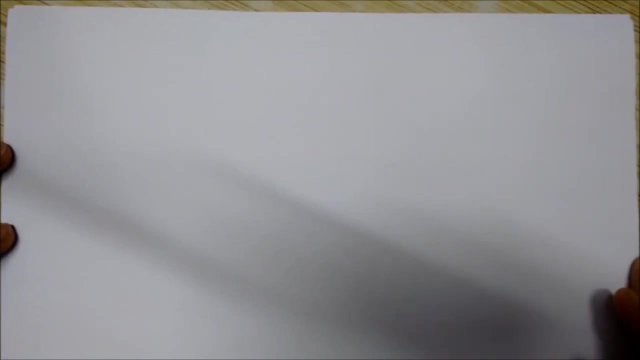 The PAM, PWM and PPM were the analog pulse modulation techniques that we have discussed. Now we will discuss the pulse code modulation, PCM. We have discussed PAM, PWM and PPM. Now we are going to discuss PCM- Pulse Code Modulation- which is the digital form of this Pulse Modulation. 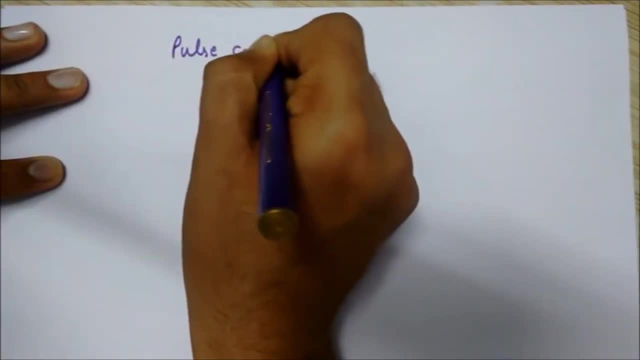 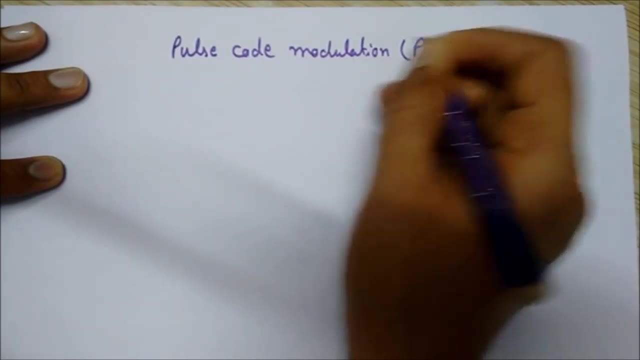 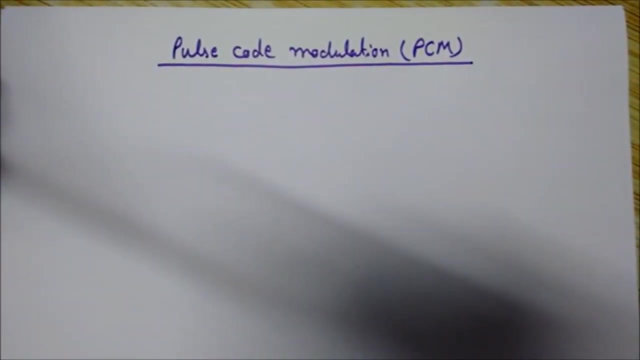 Technique known as PCM also. So what is Pulse Code Modulation? We will see. Pulse Code Modulation is a digital pulse modulation technique. PCM is a digital technology using which it is possible to transmit any analog signal in the form of binary bits. Binary means zeros and ones. For this, the 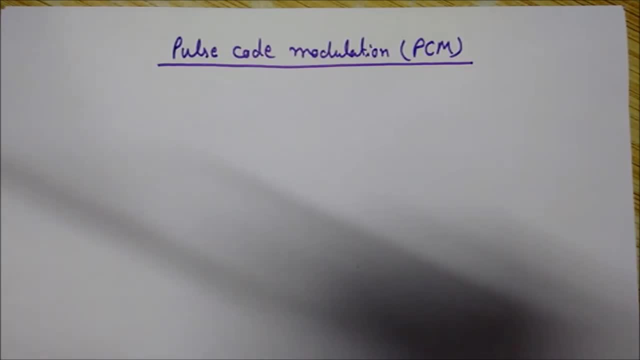 analog signal to be transmitted is first sampled using the sampling theorem. This sampled signal is quantized. The quantization is a process where the sampled signal is cut into many levels and the value of the signal is rounded off to the nearest value of the fixed level. If you are not getting 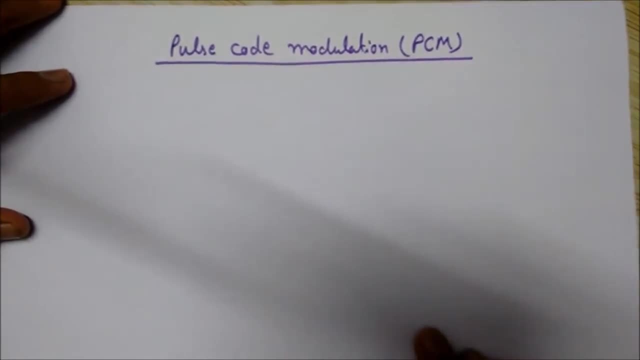 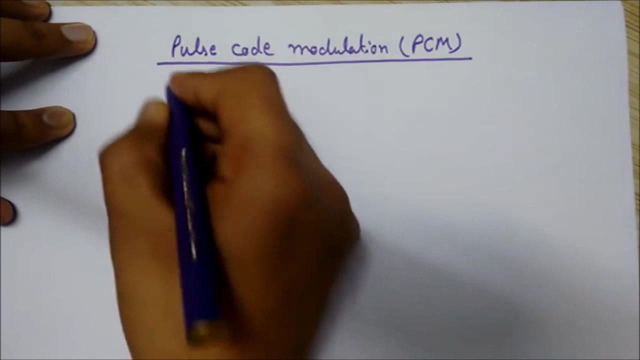 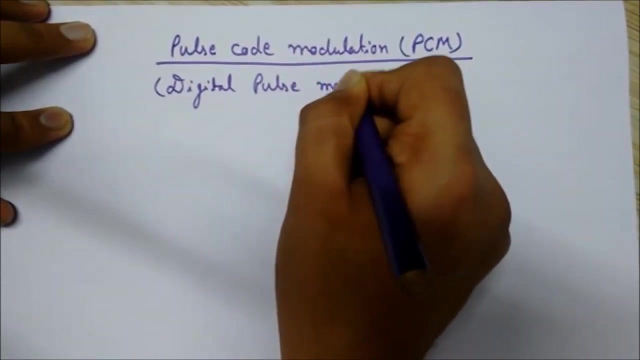 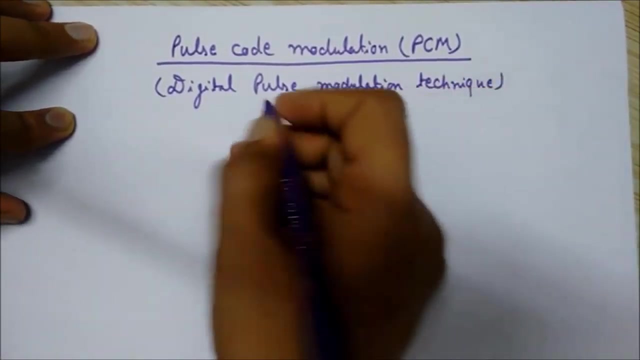 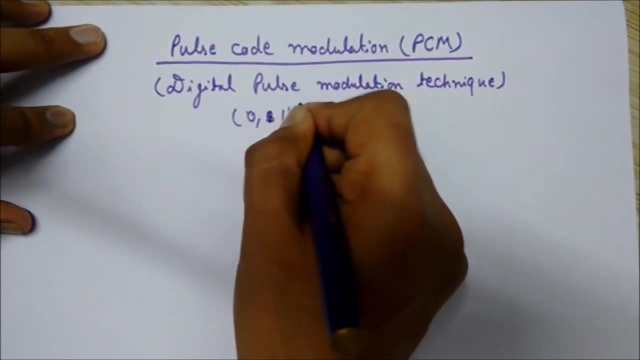 it, then I will explain it with the help of an example and diagram. So you know that Pulse Code Modulation is nothing but a digital pulse modulation technique. It is a digital pulse modulation technique. Okay, it is binary form, or you can represent the signals. 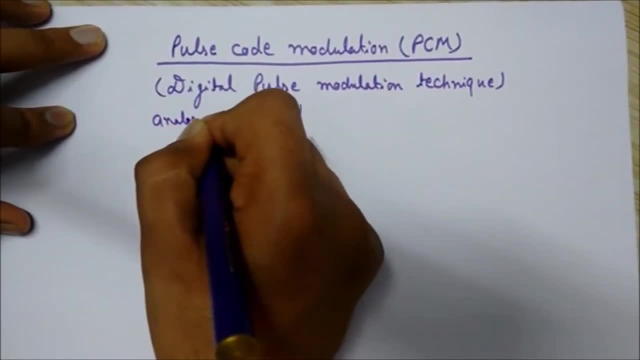 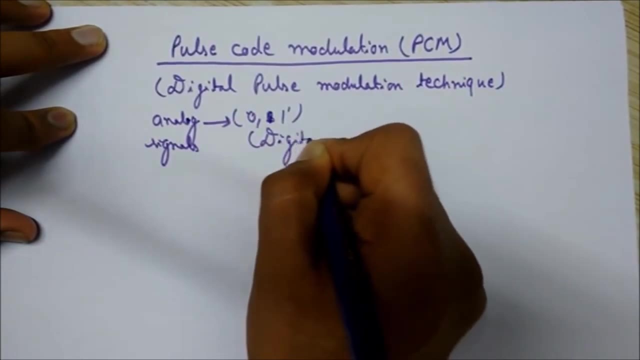 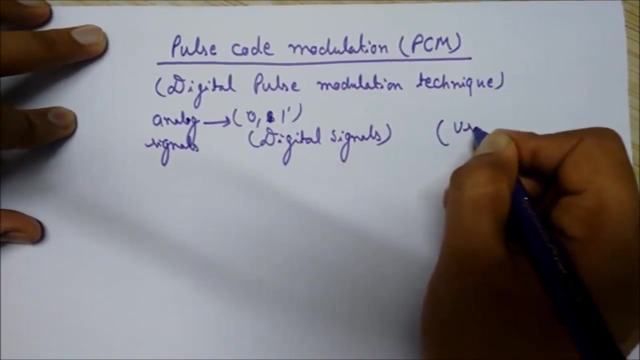 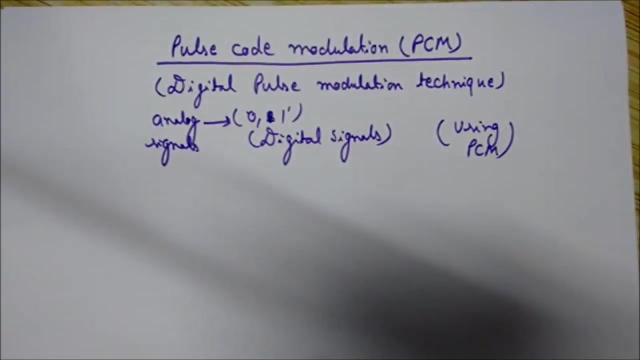 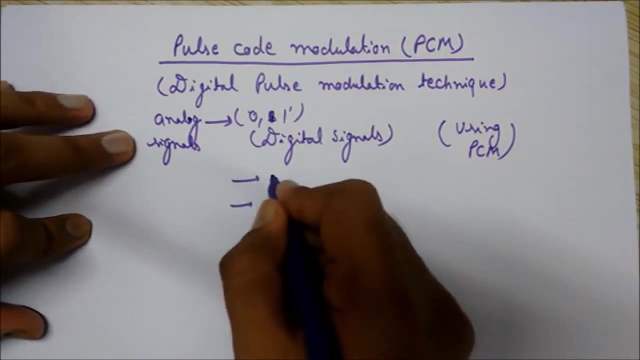 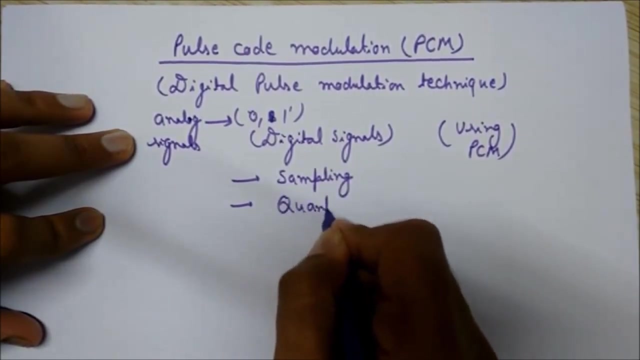 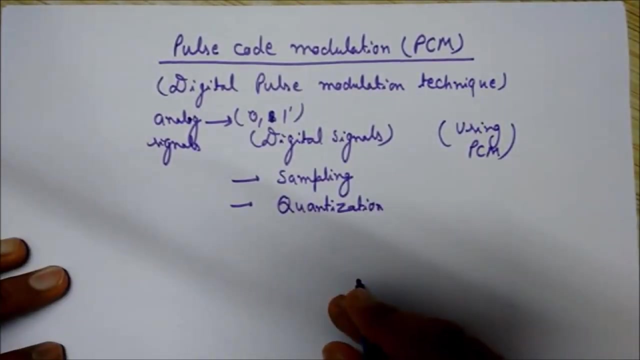 which are in analog form, Analog signals, into digital signals using PCM. Okay, using PCM, what you do? you can convert analog signals into zeros and ones. You need to use here two things: The sampling and the quantization. The sampling is based on the sampling theorem. It cuts the signal into samples. using the sampling, 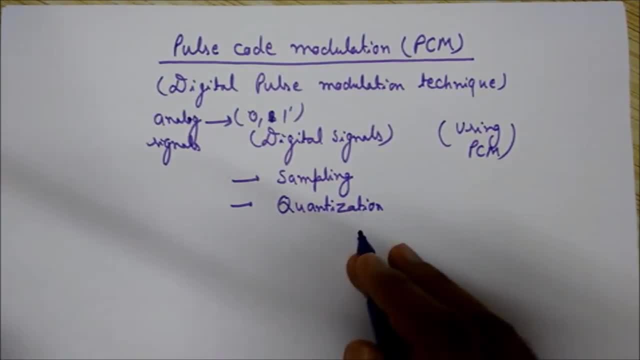 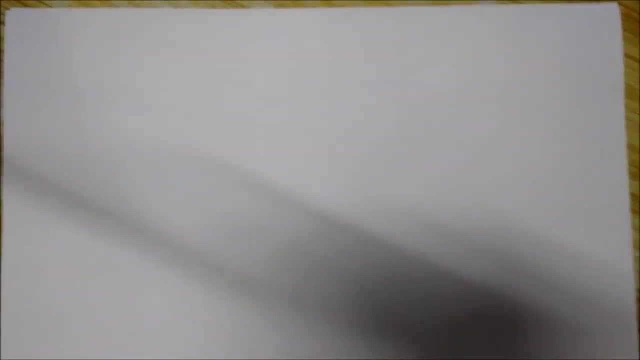 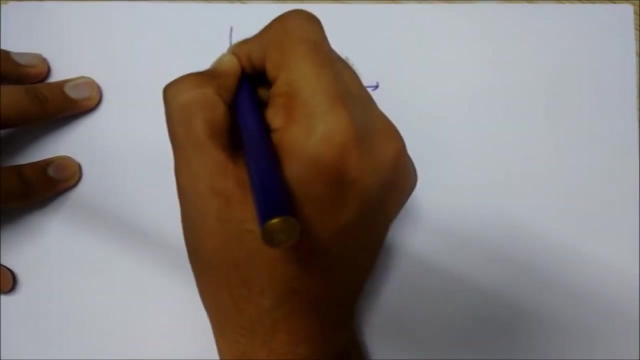 theory, theorem, and in the quantization is at the amplitude level. So to understand it we need to understand the concept of quantization and sampling. So I will draw the diagram Here. 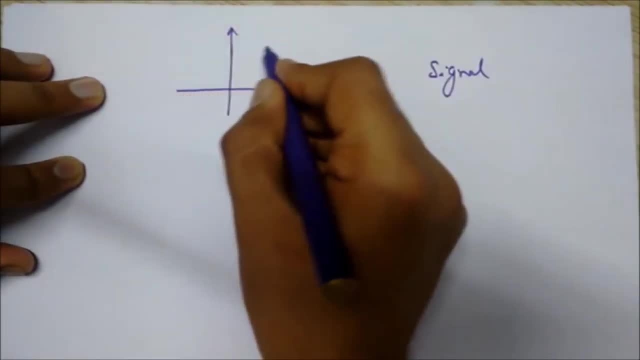 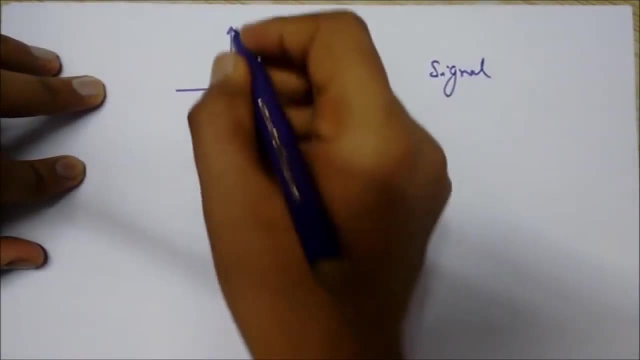 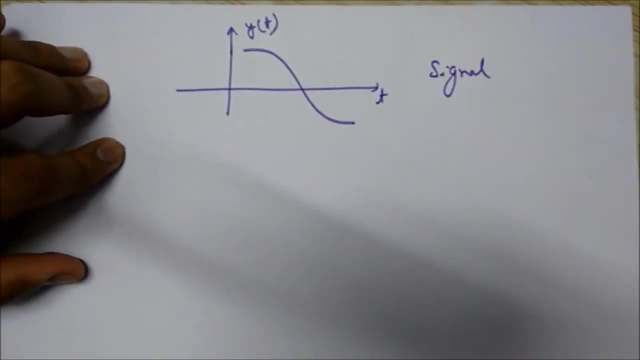 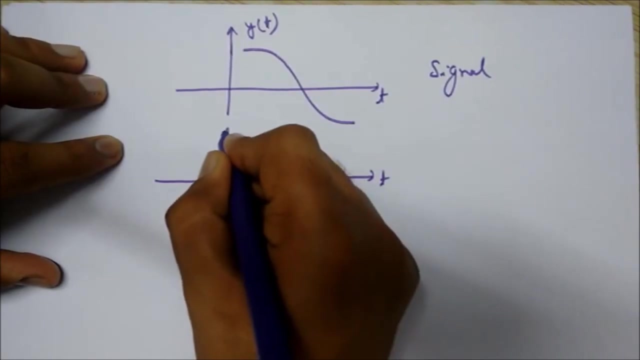 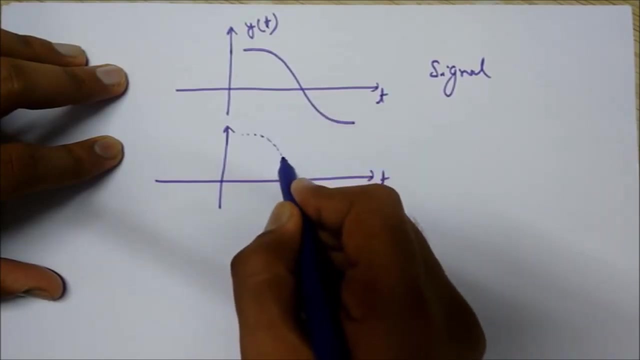 Okay, this is a signal and the time axis Let's call the signal. denote the signal with mt, And here I will sample the signal with the help of sampling theorem. So how does this look like? I'm showing it here. the sample signal is somewhat of this form. 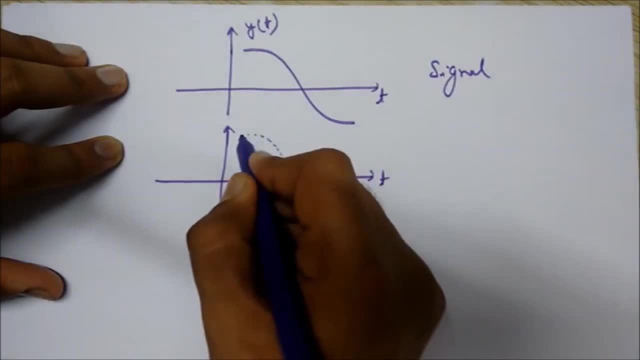 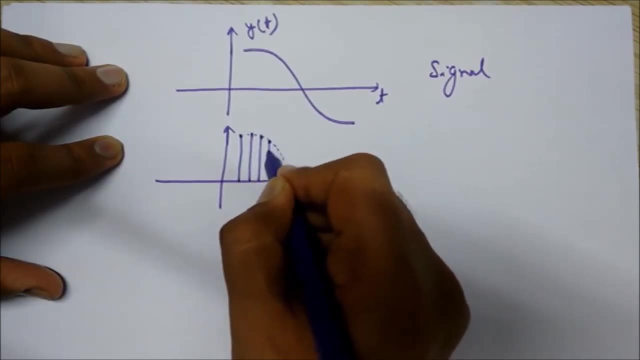 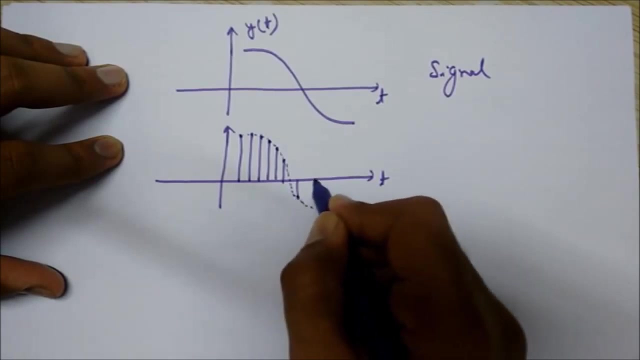 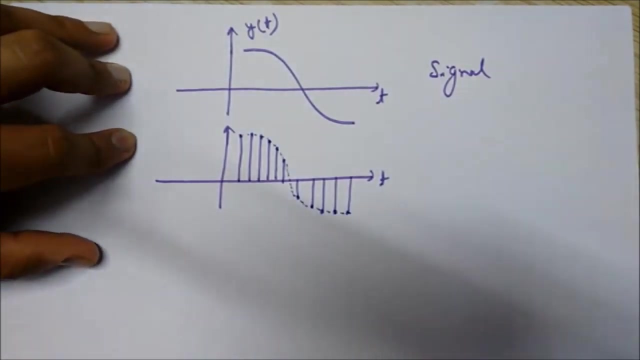 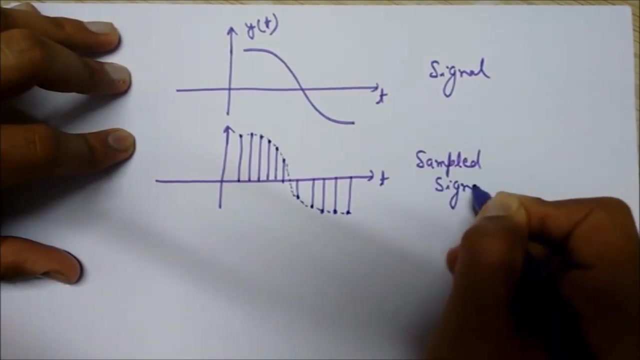 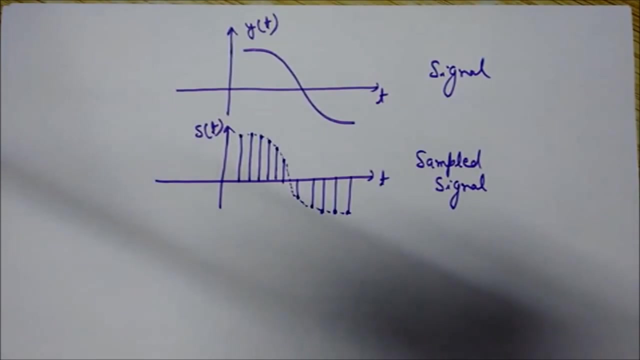 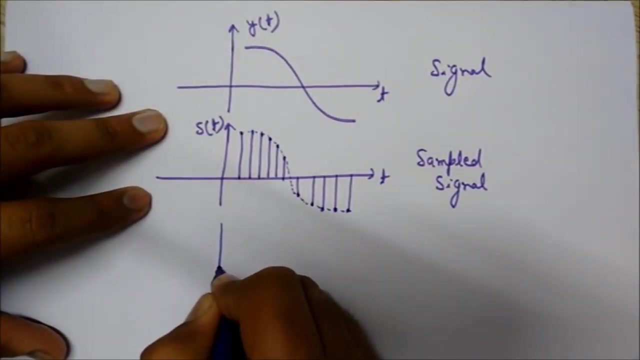 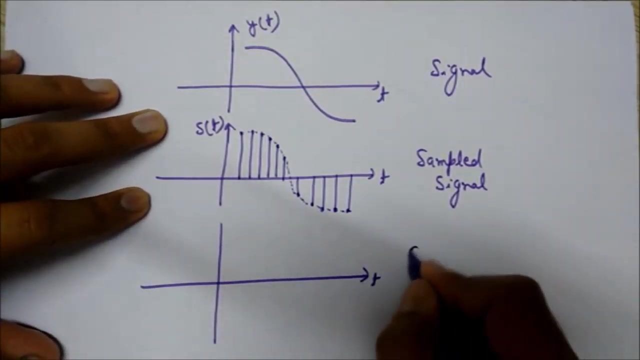 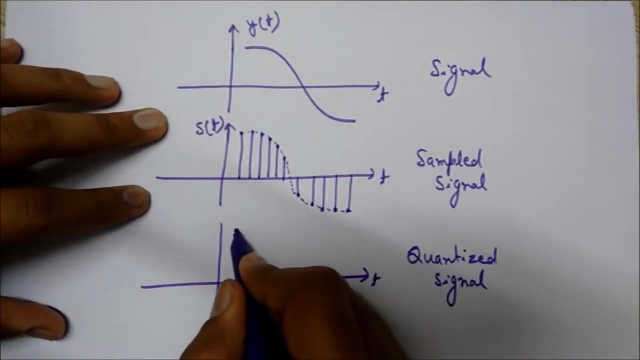 this has been cut horizontally into samples, so this is the sample signal signal. I'm denoting the sample signal with st here. now we will see the quantization process, how a quantized signal look like. so here is the quantized signal. ok, so let's see here. 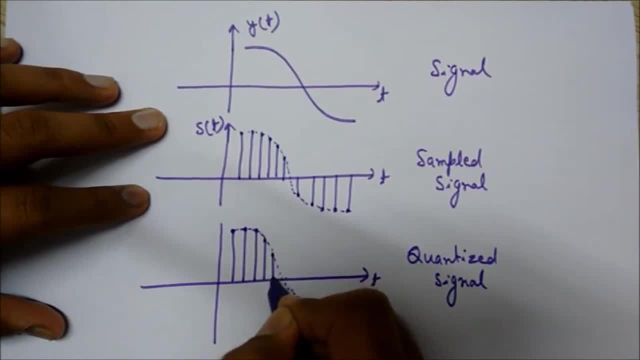 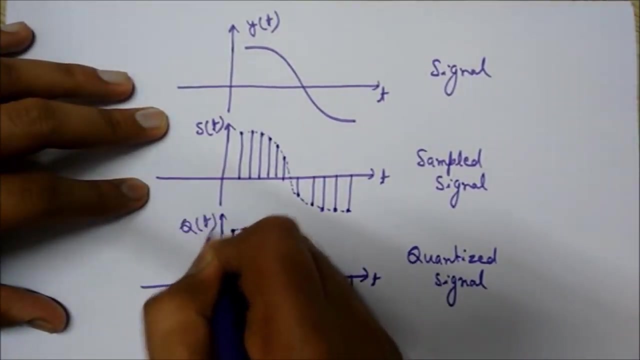 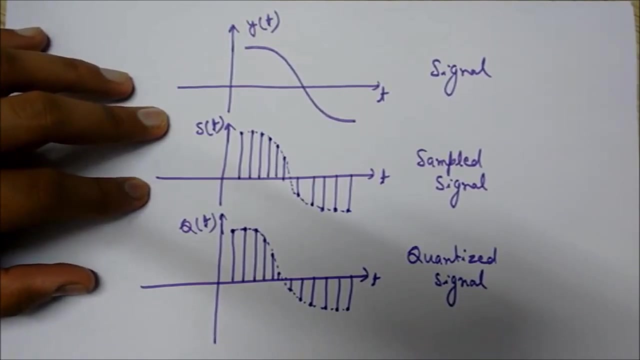 Now, if I am denoting it with Qt- quantized signal- and here is the time axis for quantization. I have already told you the definition and I have explained it earlier. what is quantization? Here we cut this amplitude into number of levels and we try to approximate the value. 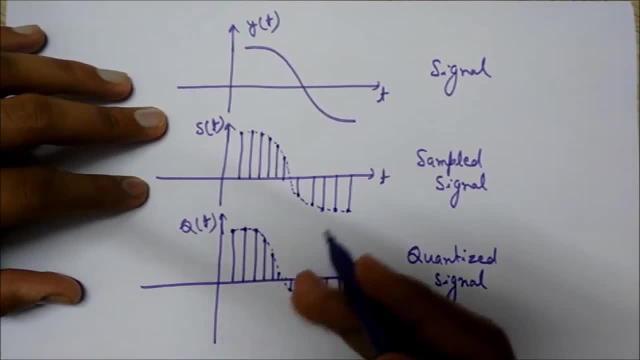 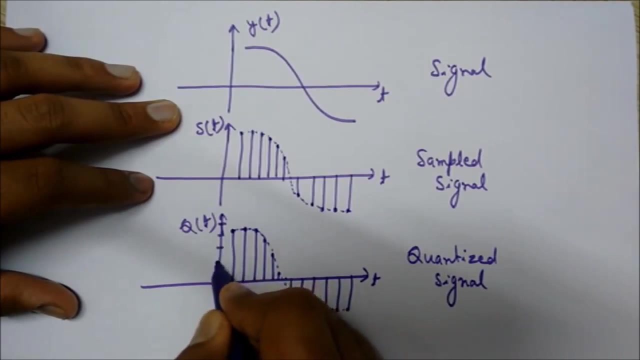 nearest to the. you can say that we try to round off the value of that signal corresponding to that fixed value of level, Fixed level value. So here I am cutting this into some levels: 1, 2,, 3,, 4,, 5,, 6,, 7,, 8.. 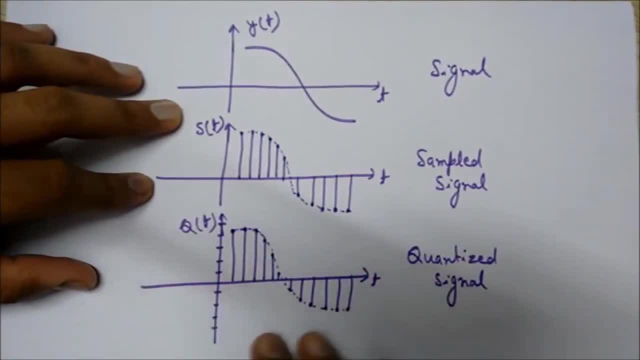 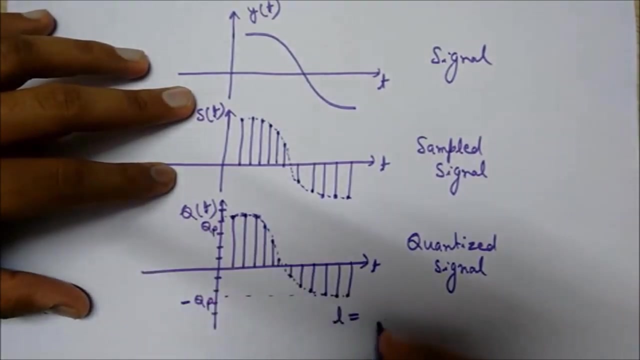 Some levels in and with the help of horizontal lines, let's say that this minimum point is minus Qp. and here is the Qp. This amplitude is 0. It's denoted by Qp. So if there are L number of levels, then L. if I am cutting it into L levels, then L is. 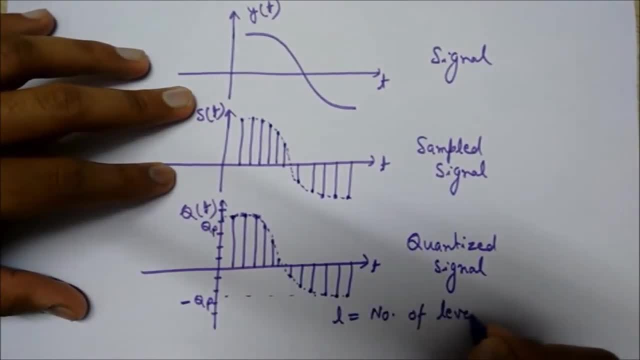 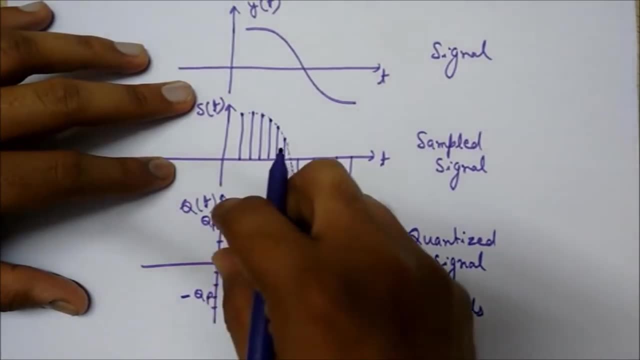 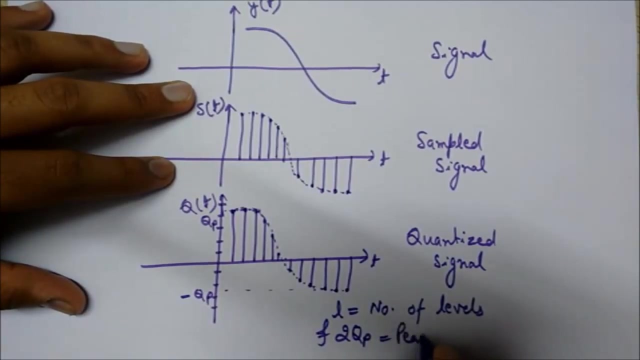 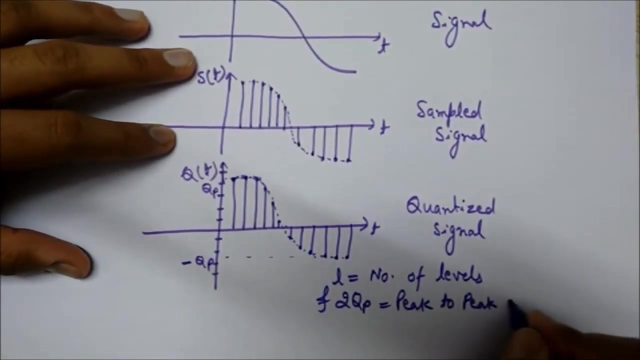 the number of levels and 2 times of Qp. you can see this is Qp, and here it is again the Qp, The Qp and Qp becomes 2Qp. Is that right? Yes, And the peak to peak amplitude: okay, which is peak to peak amplitude? and so you can. 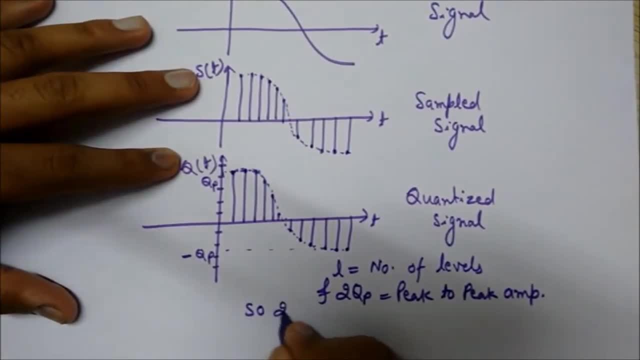 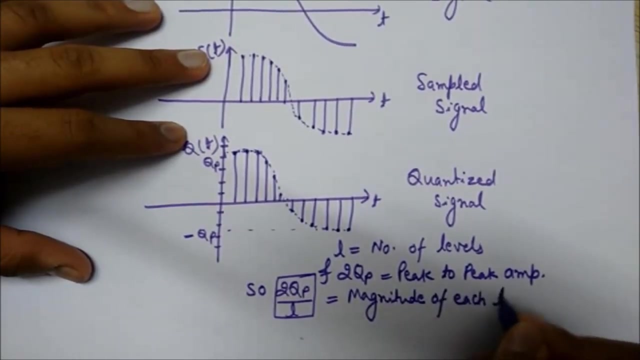 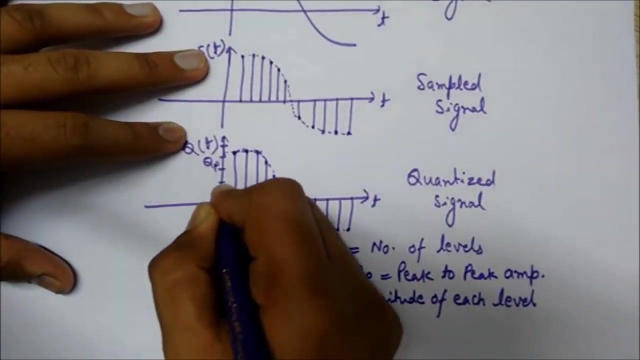 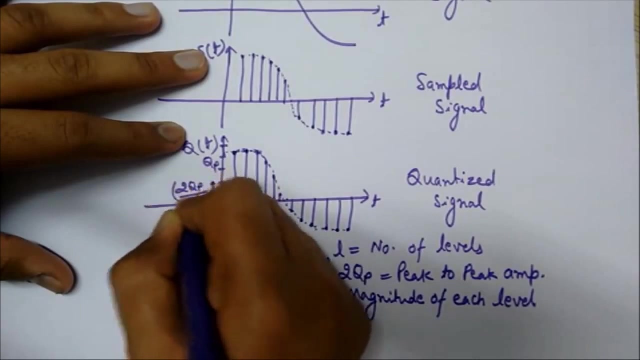 say that 2 times of Qp by L, 2 times of Qp divided by L, will be the magnitude of each level. So what is 2Qp by L or the magnitude of each level? This is the 2 times of Qp divided by L. This distance or this distance, these all are same. 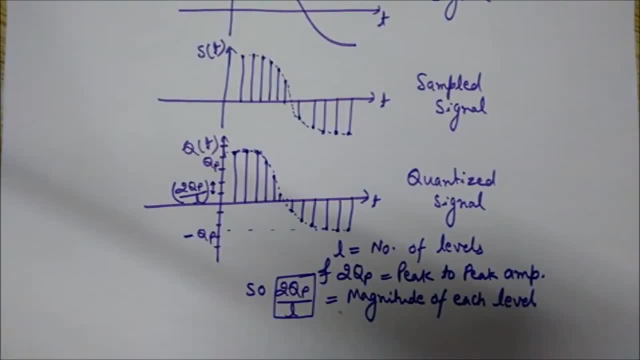 distances. So this is the 2 times of Qp divided by L. This distance or this distance, these all are same distances. So it is clear that as the number of levels increases, the accuracy of the quantized signal increases. The quantized signal is just an approximation of the original signal. 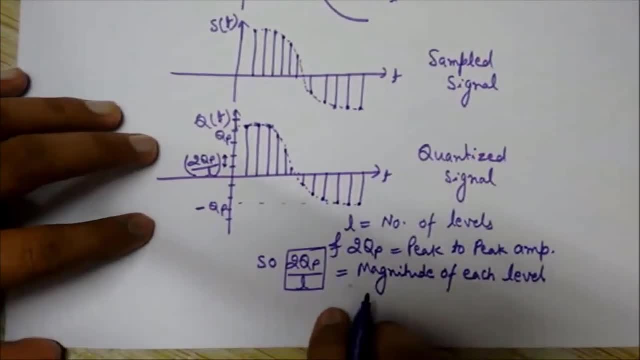 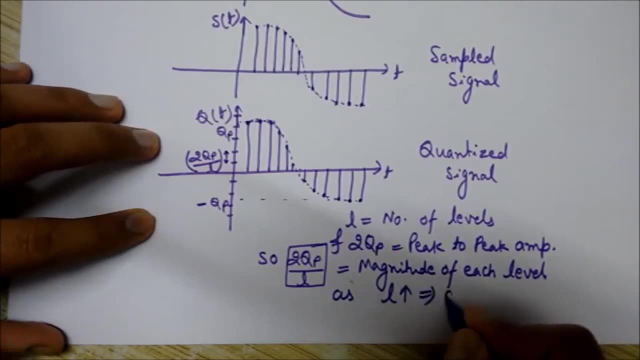 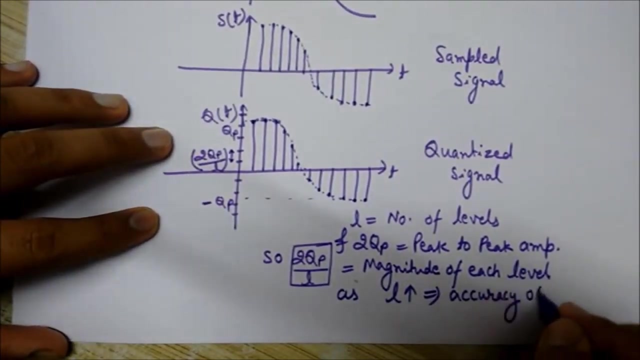 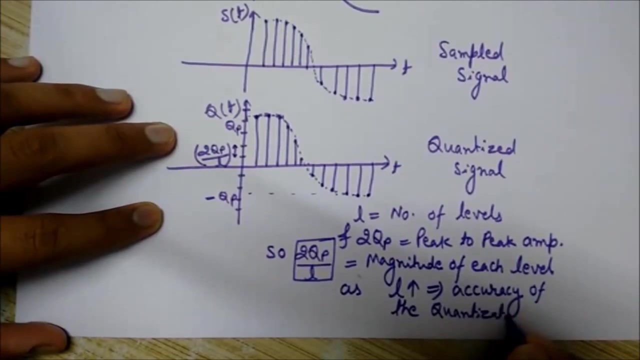 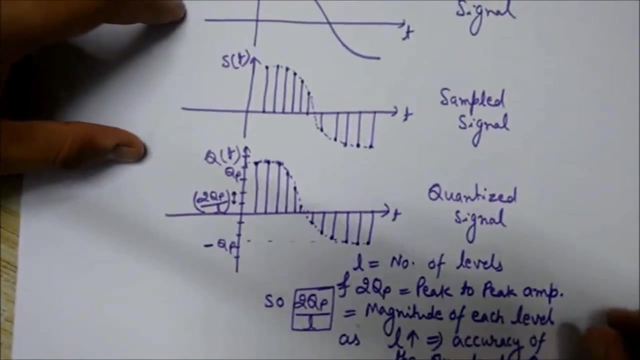 So we can say that as the number of levels increases, it implies that 2 times of Qp by L. You can see that the accuracy of the quantized signal, the quantization, also increases. So you can increase the accuracy of signal, the quantized signal, to any desired level. 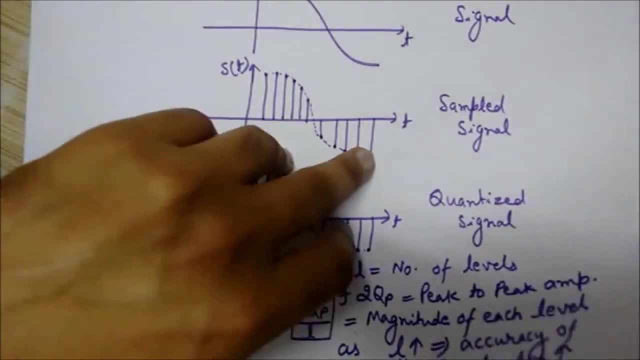 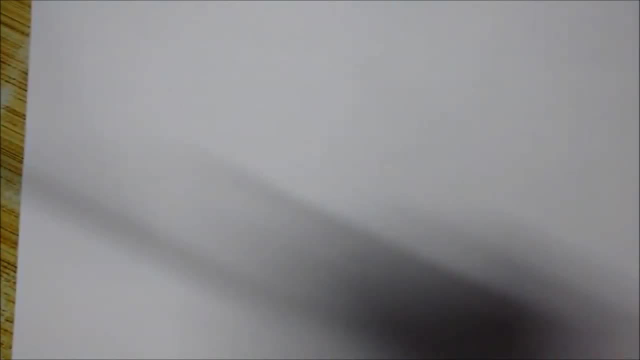 by increasing the. I need to write that I cannot. Let's start. number of levels: higher the levels. number of levels higher will be the accuracy. the pcm pulse code modulation uses this technique to convert analog signals into digital signals. now let's see. how does a pcm wave look like? i will show you now the waveform of a pcm signal.